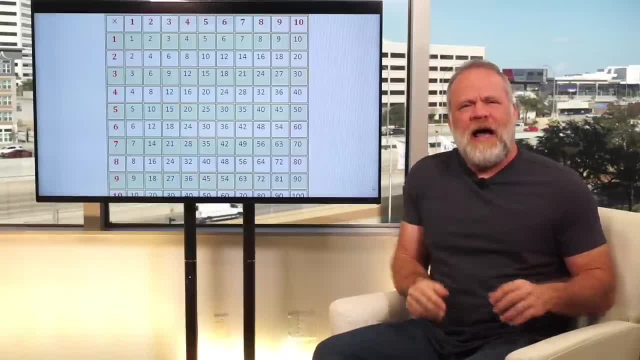 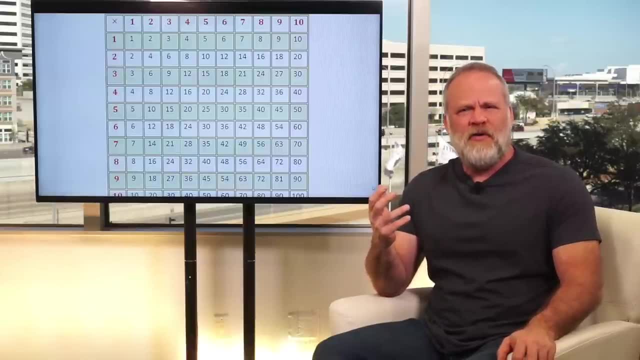 Hey guys, welcome to this video. My name is Ron White. I'm a two-time USA Memory Champion. In this video, if you are a parent and you're trying to teach your children how to memorize the multiplication tables, I'm going to walk you through exactly how I do this. when I'm trying 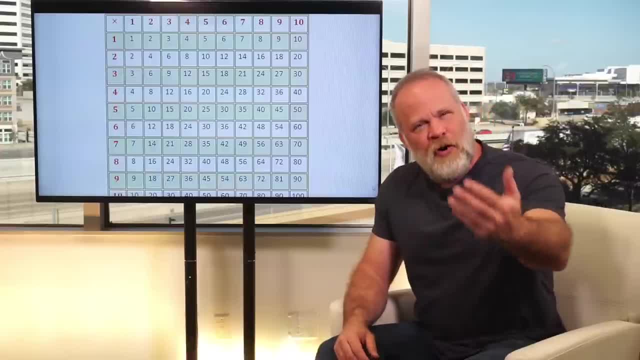 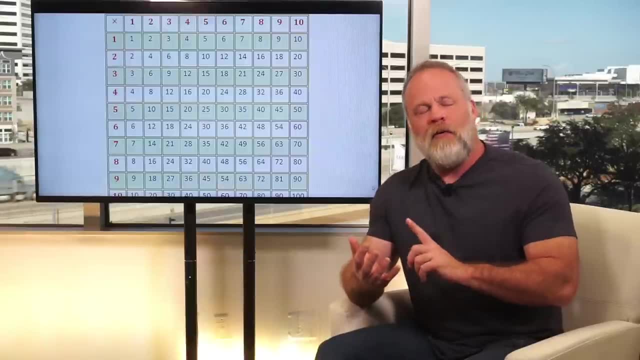 to teach someone their multiplication tables. By the way, if you enjoy my teaching style and if you want to get my Black Belt Memory course, which is going to help not just with multiplication tables but remembering what you read, studying for a test, learning foreign languages, memorizing, 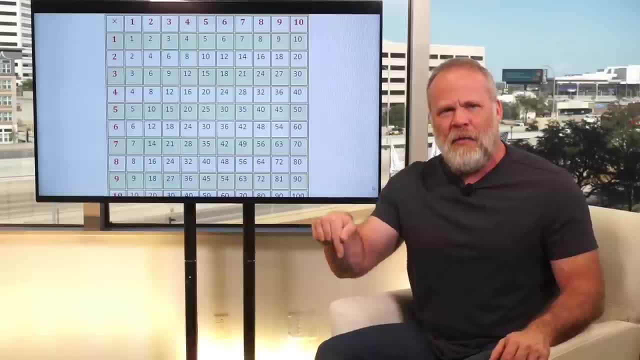 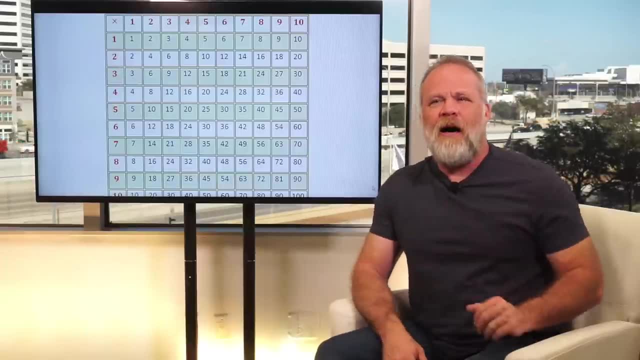 anything to get better grades as a student. click the link down below in the description. get my free memory gift and find out about my Black Belt Memory course. Now let's talk about how to memorize the multiplication tables If you're working with your child or a student on. 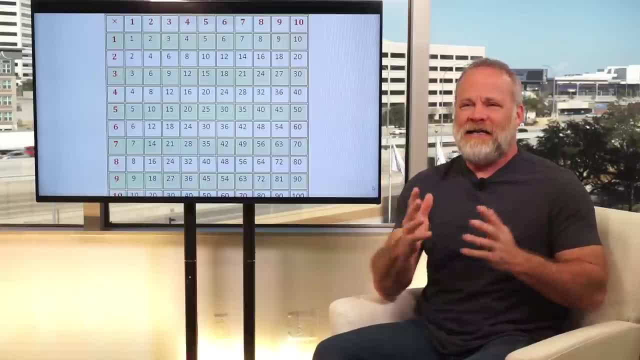 how to memorize this. it can be daunting. They look at that and they see a 10 by 10 grid. They're like, oh, there's a hundred, 10 by 10, that's a hundred different possibilities. there I got to. 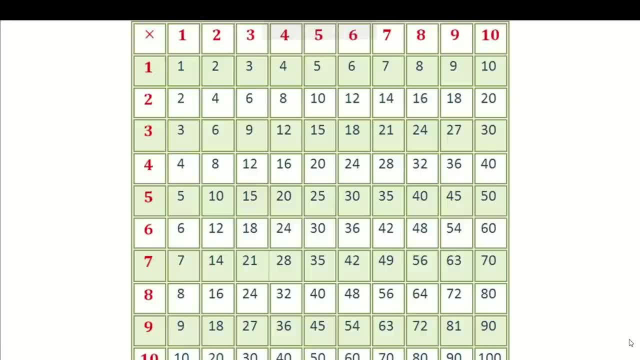 memorize them. How am I ever going to do this? Well, when we break this down, it's really not as daunting as it seems. Let's take the first one, for example, The ones. you don't really have to memorize those, do you? Because one times any number is the number One. 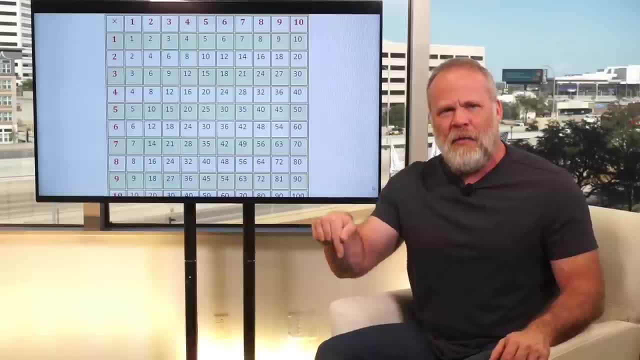 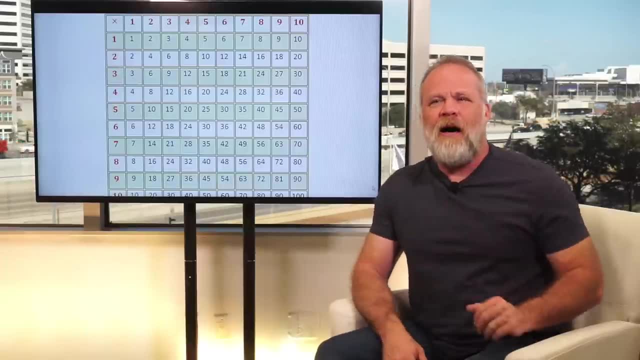 anything to get better grades as a student. click the link down below in the description. get my free memory gift and find out about my Black Belt Memory course. Now let's talk about how to memorize the multiplication tables If you're working with your child or a student on. 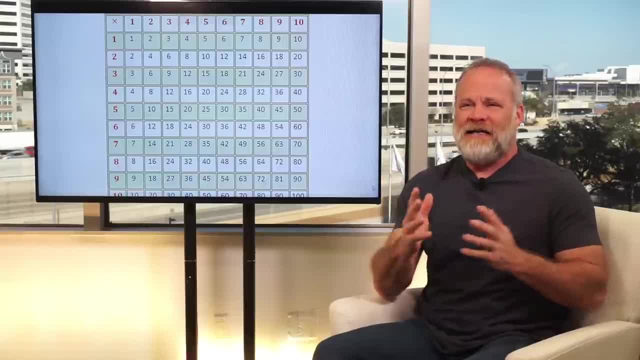 how to memorize this. it can be daunting. They look at that and they see a 10 by 10 grid. They're like, oh, there's a hundred, a hundred, 10 by 10. That's, that's a hundred different possibilities. 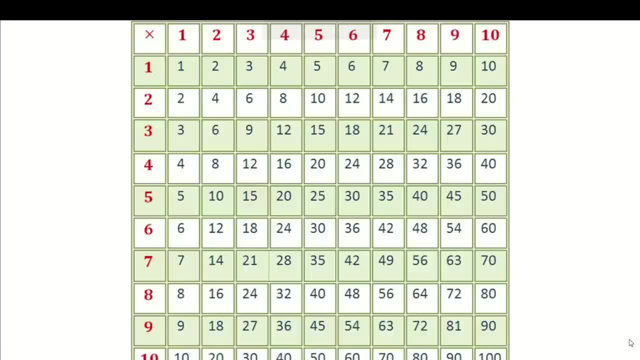 there, I got to memorize them. How am I ever going to do this? Well, when we break this down, it's really not as daunting as it seems. Let's take the first one, for example, The ones. you don't really have to memorize those, do you? Because one times any number is the number One. 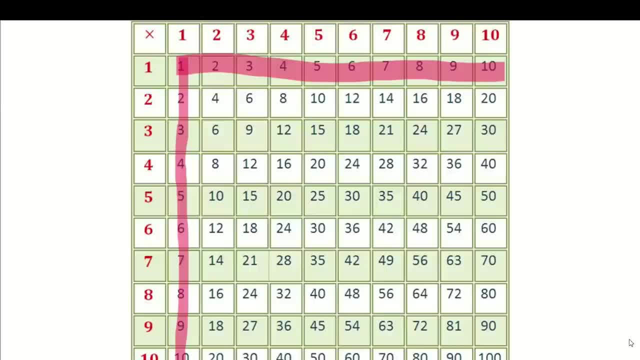 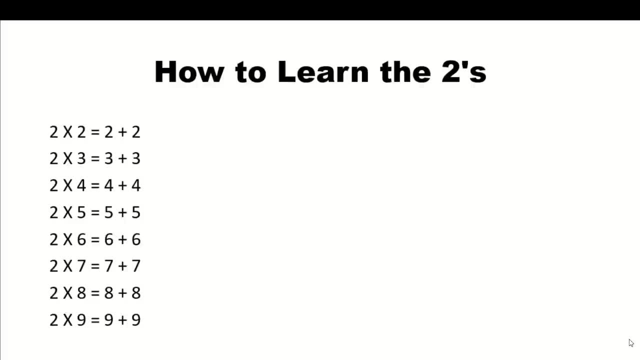 times eight is eight. One times nine is nine. So we can kind of cross those off our list. and boom, now we're down to a nine by nine grid here. Now how do we learn the twos? Now the twos. 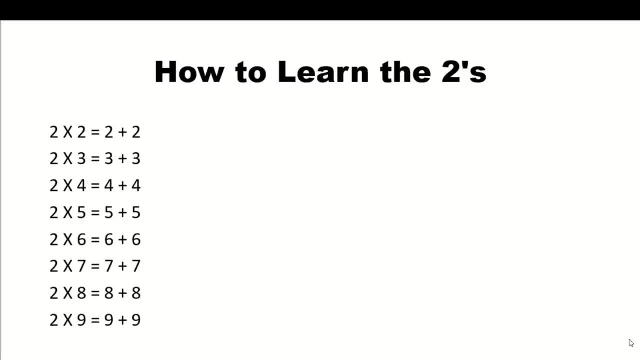 are just a multiplication problem. Two times two is two plus. If I'm working with a student, I would say what's two times three? And I would have them understand that two times three is the same as three plus three. Two times four is the same as. 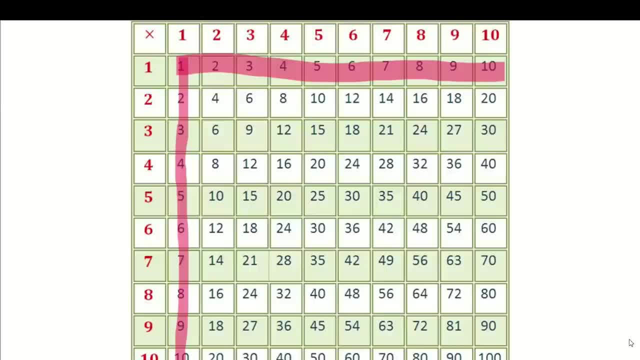 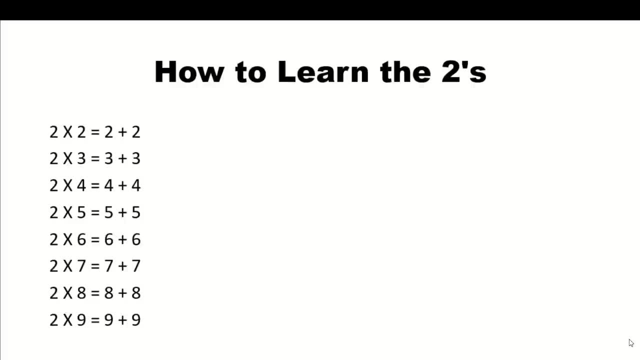 times eight is eight. One times nine is nine. So we can kind of cross those off our list. and boom, now we're down to a nine by nine grid here. Now how do we learn the twos? Now the twos. 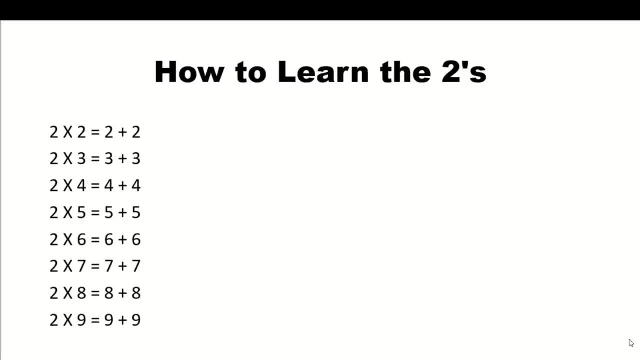 are just a multiplication problem. Two times two is two plus. If I'm working with a student, I would say what's two times three? And I would have them understand that two times three is the same as three plus three. Two times four is the same as. 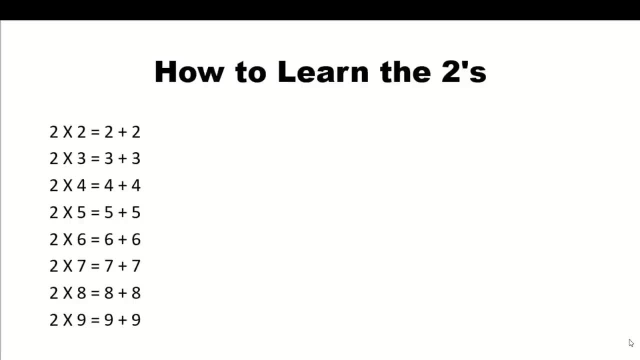 four plus four, Two times five is the same as five plus five, And have them say that and have them understand that Really, you want a student to understand the numbers. You're not wanting them to memorize it. Have them understand that two times six is six plus six. 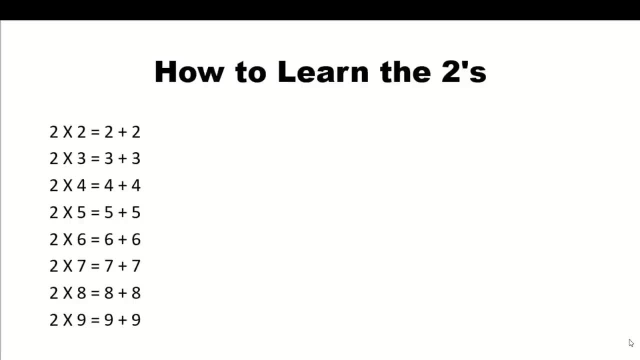 four plus four, Two times five is the same as five plus five And have them say that and have them understand that. Really want a student to understand the numbers. You're not wanting them to memorize it. Have them understand that two times six is six plus six. 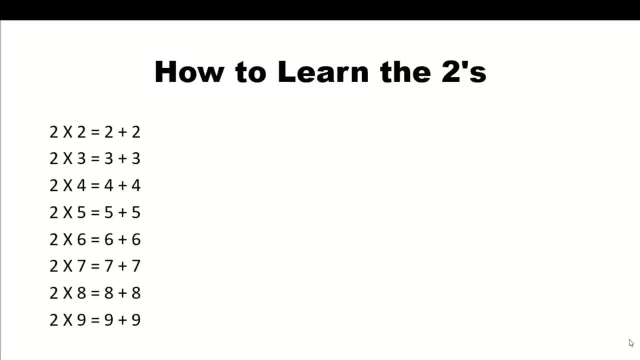 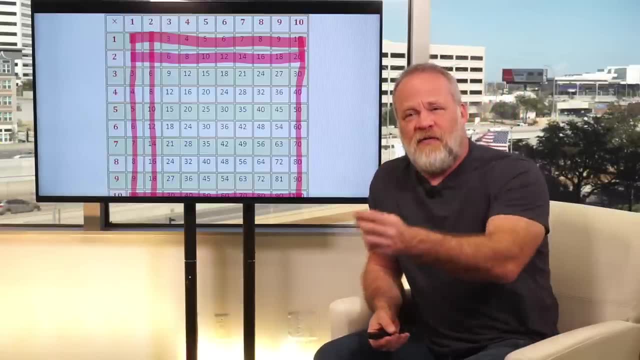 Seven is seven plus seven. This is something about the twos. Then after they do that, have them count by twos. After they really understand that two times four is four plus four, and you've got them understanding that, then have them count by twos. Two, four, six, eight. 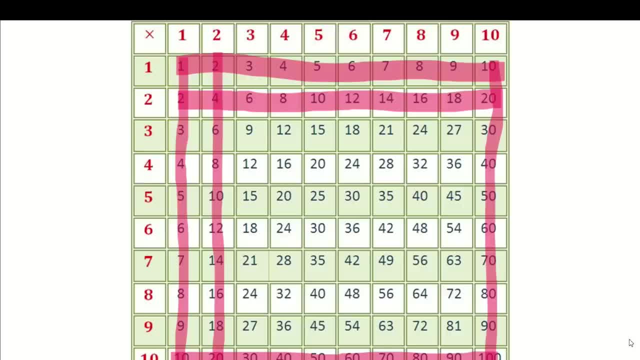 10,, 12,, 14,, 16,, 18, 20.. When they can count by twos and understand that two times five is five plus five, the twos are so easy to learn. So the ones and the twos are so easy to learn. 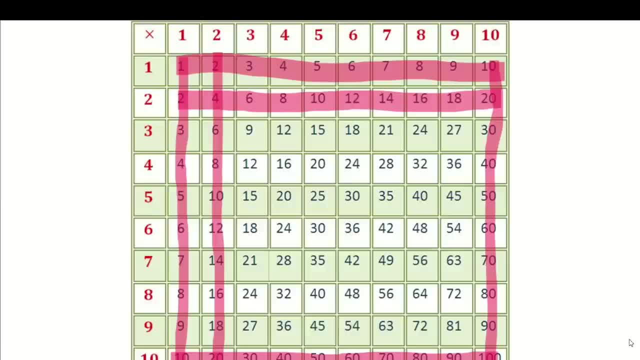 so now we can cross off all of those. Now, right, there we are down to a smaller square that we're trying to memorize. Now we're on to the threes. How would I teach a child to memorize the threes? 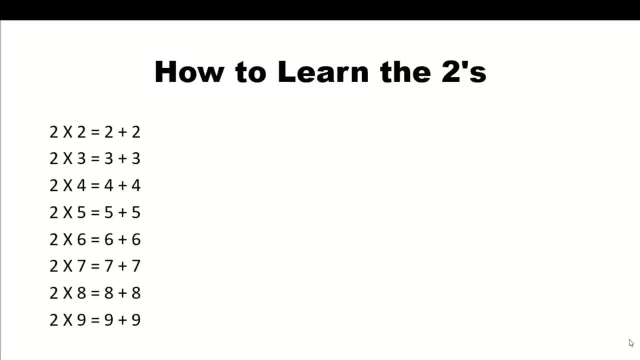 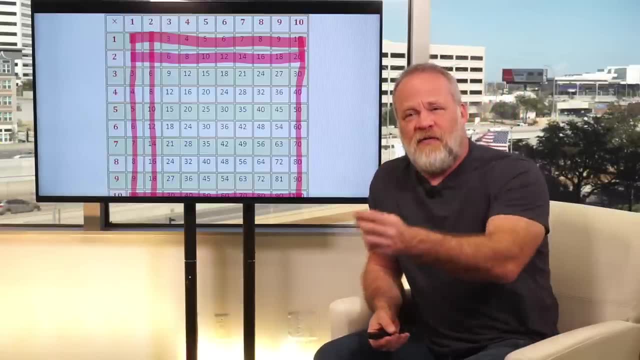 Seven is seven plus seven. This is something about the twos. Then after they do that, have them count by twos. After they really understand that two times four is four plus four, and you've got them understanding that, then have them count by twos. Two, four, six, eight. 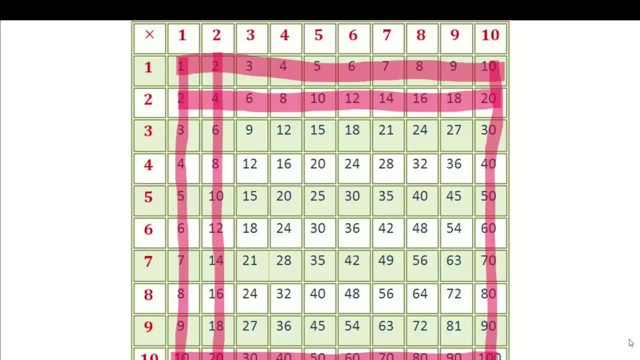 10,, 12,, 14,, 16,, 18, 20.. When they can count by twos and understand that two times five is five plus five, the twos are so easy to learn. So the ones and the twos are so easy to learn. 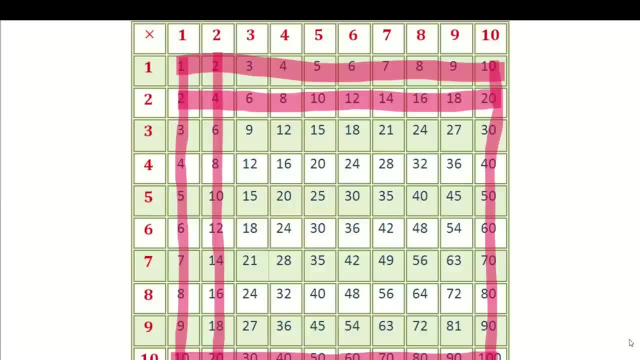 so now we can cross off all of those. Now, right, there we are down to a smaller square that we're trying to memorize. Now we're on to the threes. How would I teach a child to memorize the threes? 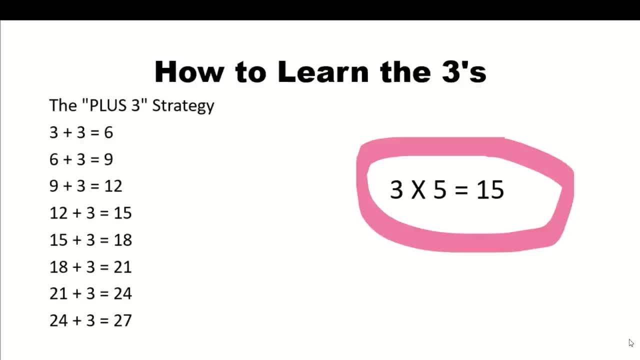 I use the plus three strategy. So three plus three is six. And then I would say to the child: plus three and they would say nine. Then I would say plus three and they would say 12.. Plus three and they would say 15.. I would say: 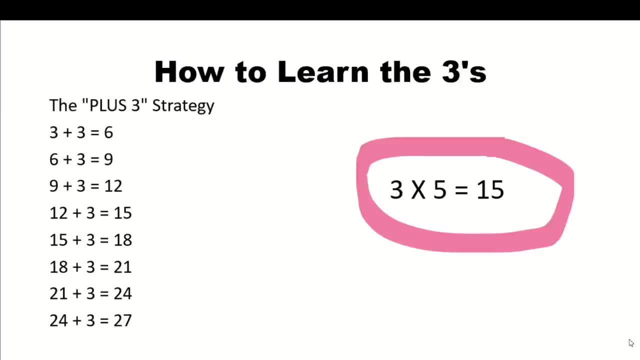 three and they would say 18. Plus three, and then they would say 21.. Plus three and they would say 24. Plus three and they would say 27.. Once you can get them to see the plus three strategy, you're just adding three to the last one. have them understand it, Remember. 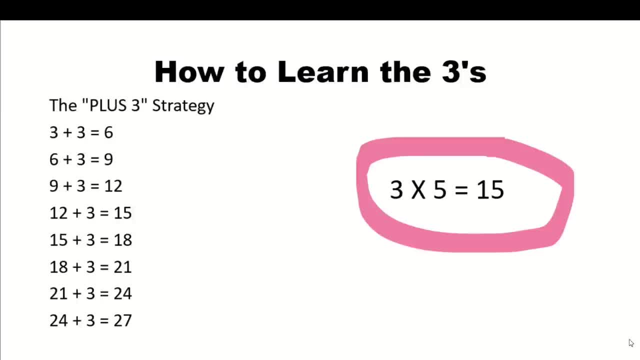 understanding is the key here. Then, once they understand that, then do the counting real fast again: Three, six, nine, 12,, 15,, 18,, 21,, 24,, 27,, 30. Have them do the counting fast and then they've. 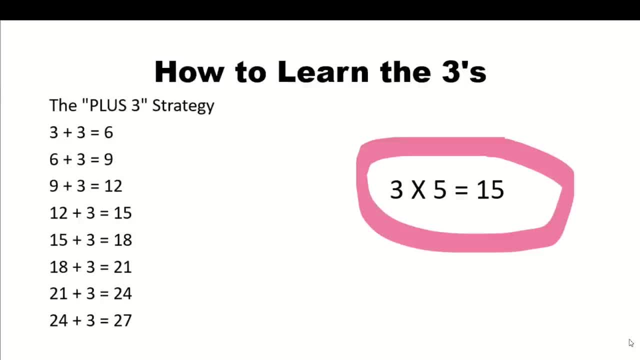 got to do the threes. I always like to just have a middle ground test there and say what's three times five then, And they will say 15, because the fives are easy. The fives always end in a zero or a. 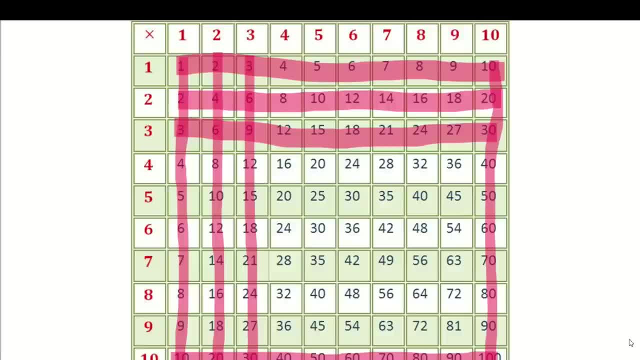 five. Now you can cross out all the threes. Now you've crossed off all the ones, all the twos, all the threes, and now you're down to a six by six square. here. This isn't really that daunting if you break it down this way. How to learn the fours, I do it the same strategy as on how to 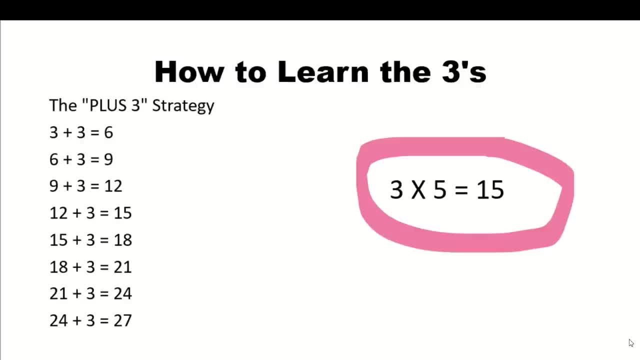 I use the plus three strategy. So three plus three is six. And then I would say to the child: plus three and they would say nine. Then I would say plus three and they would say 12.. Plus three and they would say 15.. I would say plus. 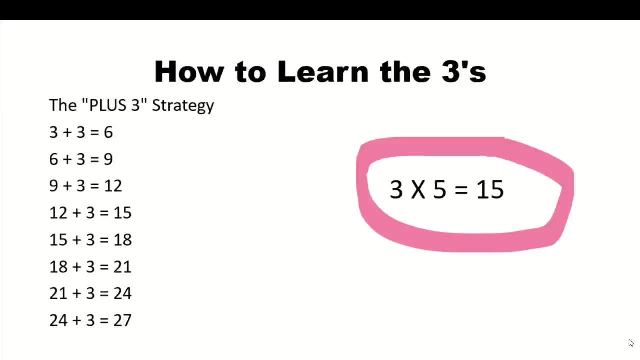 three and they would say 18. Plus three, and then they would say 21. Plus three and they would say 24. Plus three and they would say 27.. Once you can get them to see the plus three strategy, you're just adding three to the last one. have them understand it, Remember understanding. 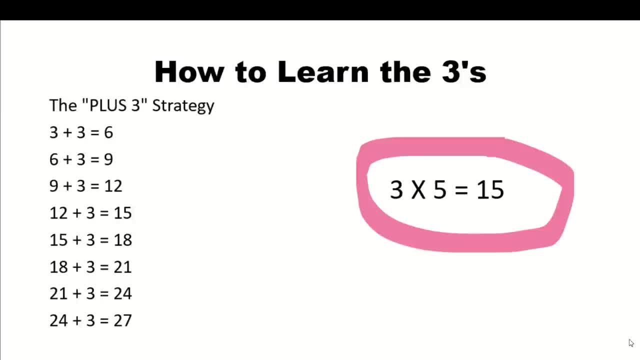 is the key here. Then, once they understand that, then do the counting real fast again: Three, six, nine, 12,, 15,, 18,, 21,, 24,, 27,, 30. Have them do the counting fast, and then they've mastered. 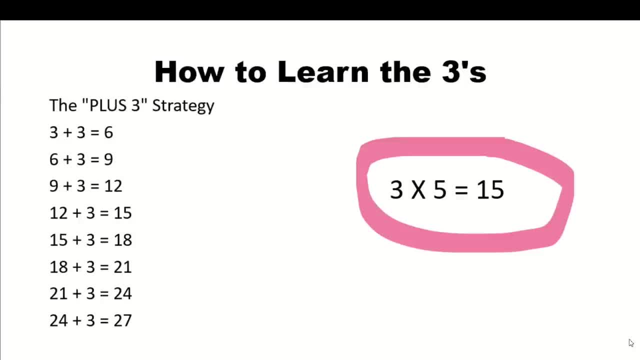 the threes. I always like to just have a middle ground test there and say: what's three times five then? And they will say 15, because the fives are easy. The fives always end in a zero or a five. 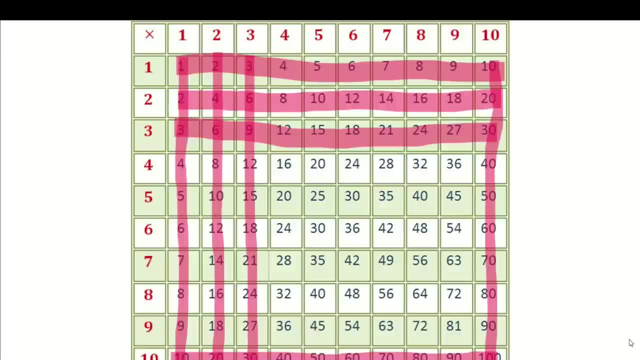 Now you can cross out all the threes. Now you've crossed off all the ones, all the twos, all the threes, and now you're down to a six by six square here. This isn't really that daunting if you break it down this way. How to learn the fours, I do it the same strategy as on how to 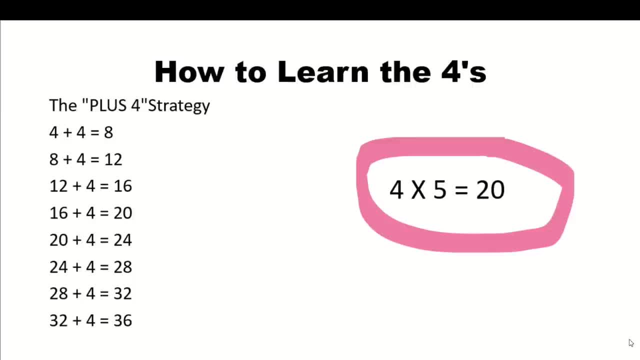 learn the threes, I do this with a plus three strategy. I do it the same strategy as on how to learn the fours. I do this with a plus four strategy. I say: what's four plus four? They say eight plus four, 12, plus four, 16, plus four, 20, plus four, 24, plus four, 28, plus four, 32,. 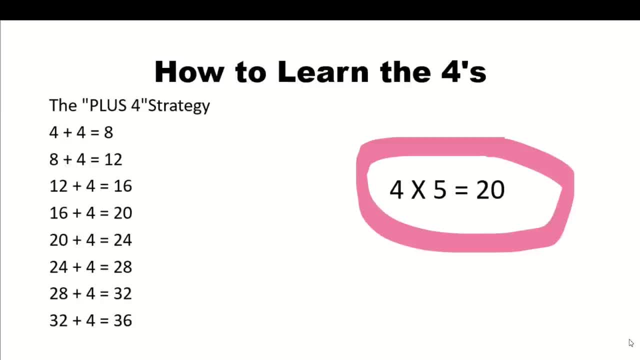 plus four, 36.. Have them understand that you're adding four each time. And then, once they've gotten real good at that, then maybe you can say: hey, can you count by fours? Four, eight, 12,, 16,, 20,, 24,, 28,, 32,, 36,, 40. Then I will just sometimes randomly throw in there: what's four? 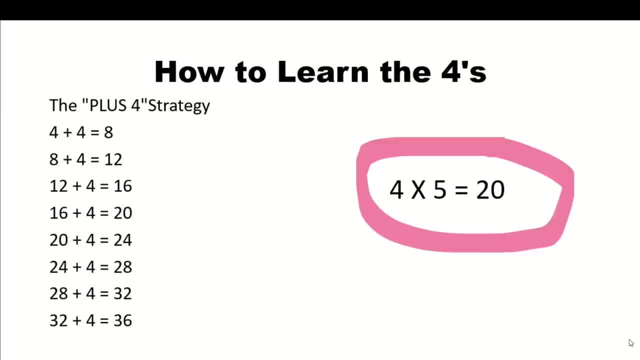 times five, And they'll say 20, because again, that's an easy one: It's either going to end in a zero or it's going to end in a five. I like knocking the fives out of the way. Why do I like doing that so much? 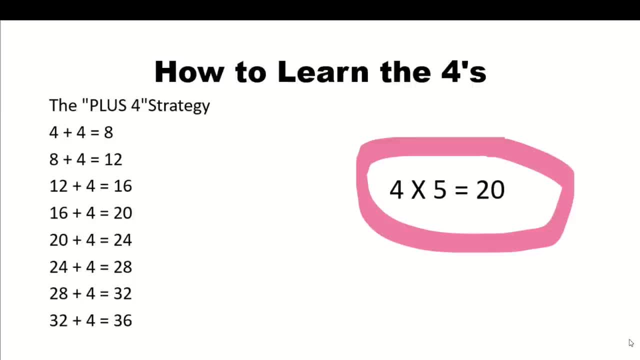 learn the threes. I do this with a plus three strategy. I do it the same strategy as on how to I say what's four plus four. They say eight plus four, 12, plus four, 16, plus four, 20, plus. 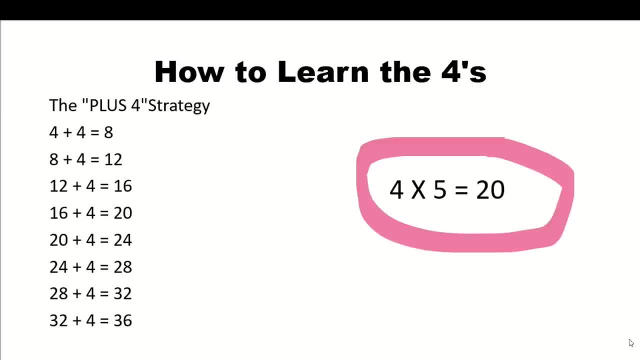 four 24, plus four 28, plus four 32, plus four 36.. Have them understand that you're adding four each time And then, once they've gotten real good at that, then maybe you can say hey, can you? 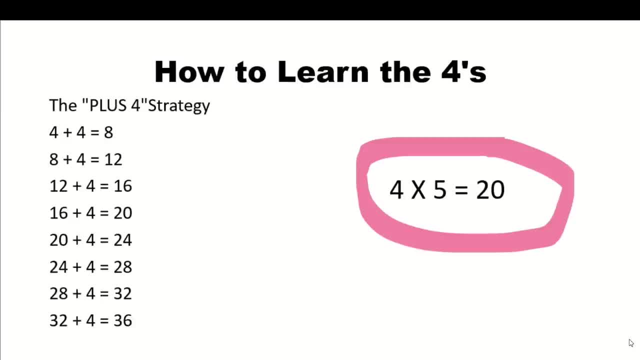 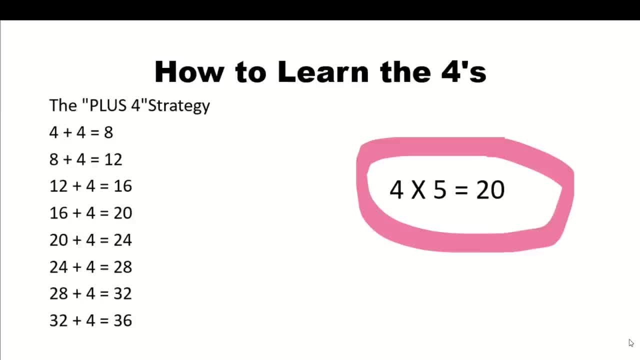 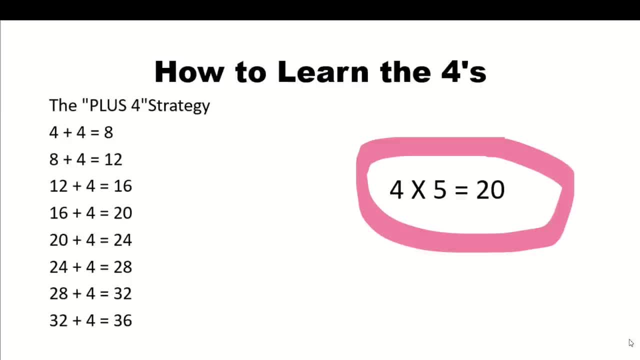 end in a five. I like knocking the fives out of the way. Why do I like doing that so much? Well, we're going to see here in a minute. Now we've crossed off the ones, the twos, the threes. 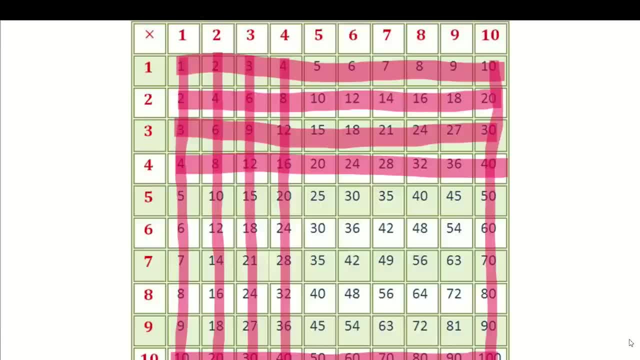 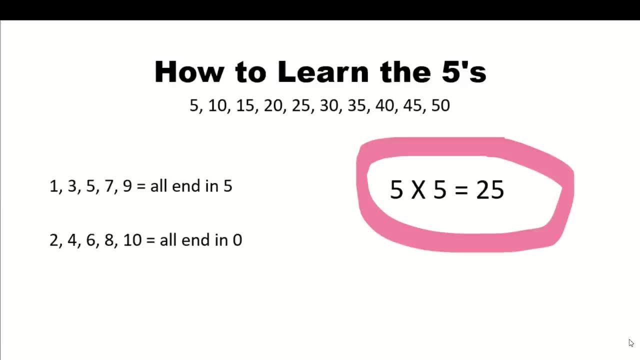 and the fours. Now we're down to a little bitty five by five section. there And again we're onto the fives right now. right, The fives are easy. Anybody can count by fives. five: 10, 15,, 20,, 25,, 30,, 35,, 40,, 45,, 50. Matter of fact, have them count by fives. 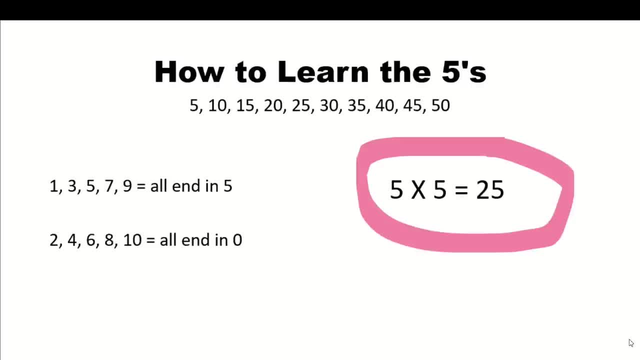 And here is a thing that you can tell your student to check their work. The odds one, three, five, seven, nine, they're all going to end in five. The evens two, four, six, eight, 10, they're all going to end in zero. So all the odds end in five. All the evens end in zero, Five. 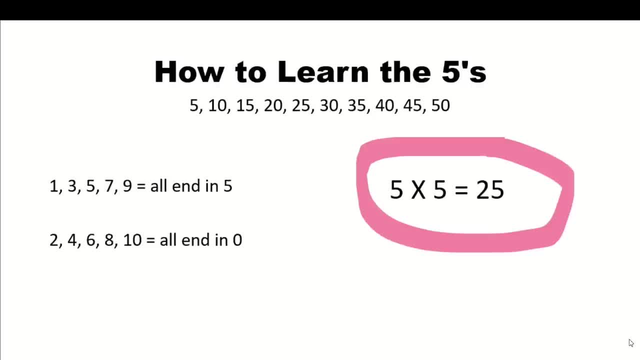 times six is 30.. Five times eight is 40.. Five times 10 is 50. And again I always go back to the middle one. Five times five is 25.. And then just have them count by fives And once they do, 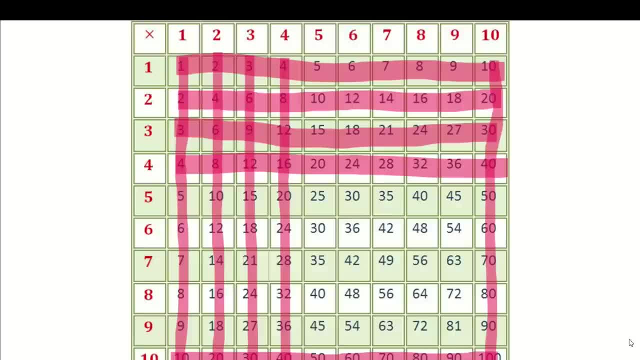 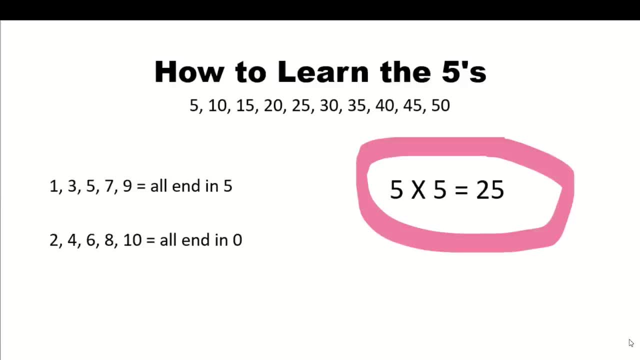 Well, we're going to see here in a minute. Now we've crossed off the ones, the twos, the threes and the fours. Now we're down to a little bitty five by five section there, And again we're onto the fives. right now, right. 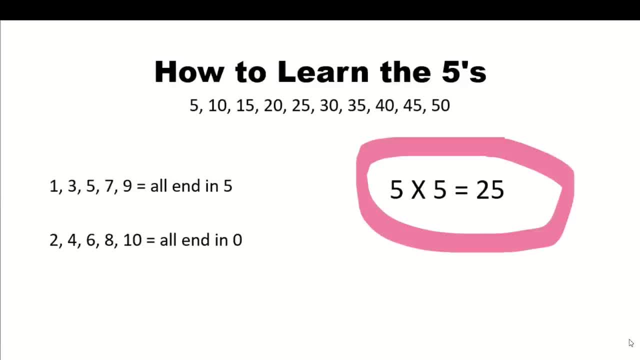 The fives are easy. Anybody can count by fives. five, 10,, 15,, 20,, 25,, 30,, 35,, 40,, 45,, 50. Matter of fact, have them count by fives. 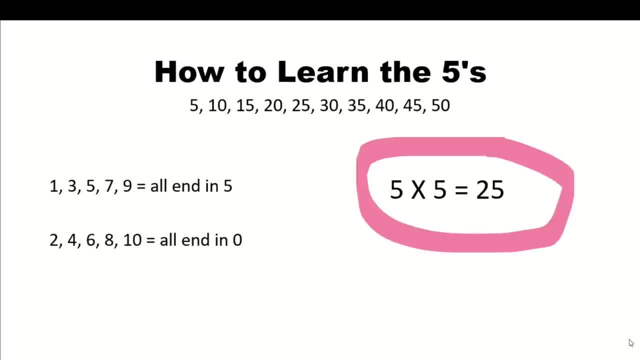 And here is a thing that you can tell your student to check their work: The odds one, three, five, seven, nine, they're all going to end in five. The evens two, four, six, eight, 10,. they're all going to end in zero. 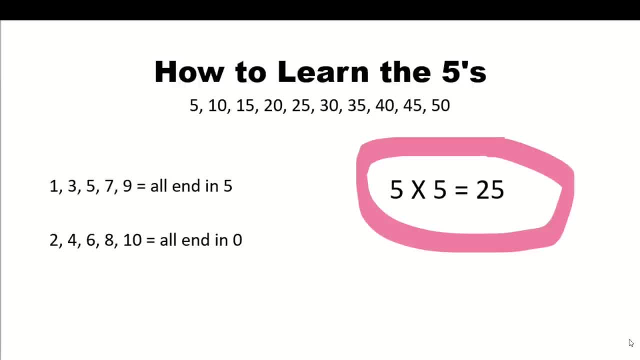 So all the odds end in five, All the evens end in zero. Five times six is 30.. Five times eight is 40.. Five times 10 is 50. And again I always go back to the middle. one. Five times five is 25.. 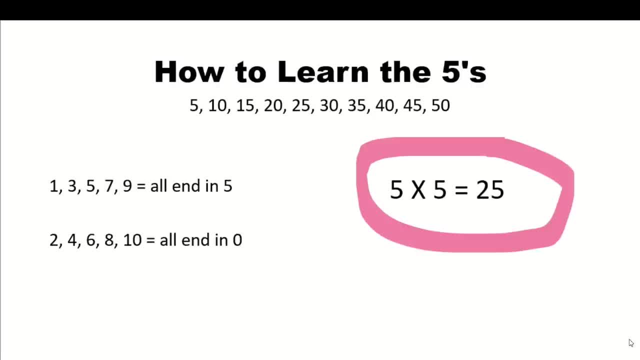 And then just have them count, Counting by fives, and once they do that, they've knocked the fives out. You're going to see that counting by twos, counting by threes, is something that can ingrain that pattern in their mind. 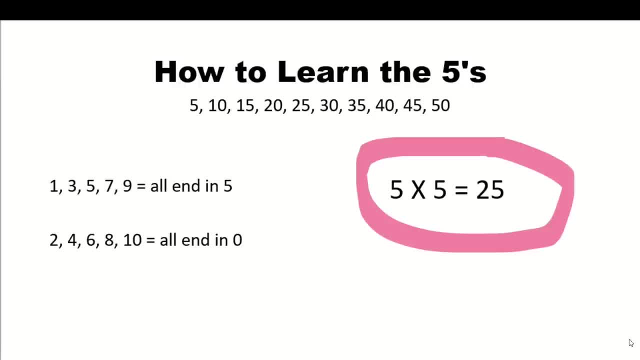 They can recognize it. But I always like to do the plus three strategy or plus four strategy so they can see you're just adding that number to get the next number. And again I'll always say what's five times five, Because it's the middle one, 25.. 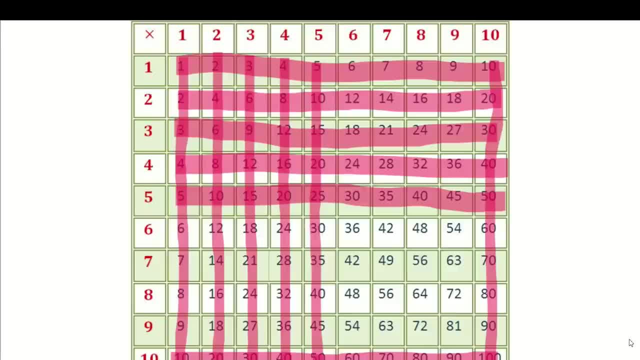 Once you've done that, the ones were easy, the twos were easy, the threes were easy, the fours were easy, The fives are easy. Now we are down to a four by four square here, And this is all we have to memorize now. 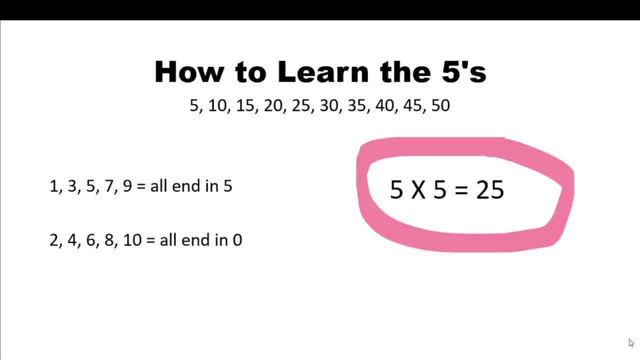 that they've knocked the fives out. You're going to see that counting by twos, counting by threes, is something that can ingrain that pattern in their mind. They can recognize it. But I always like to do the plus three strategy or plus four strategy so they can see you're just adding that. 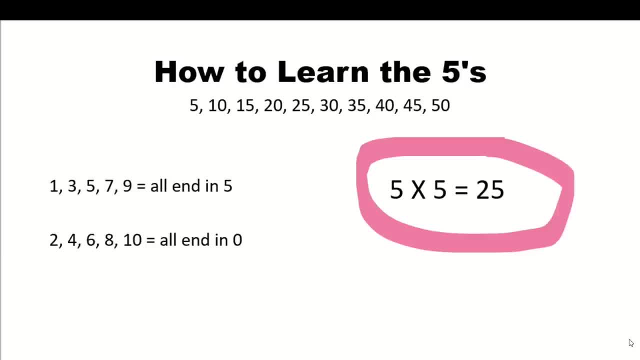 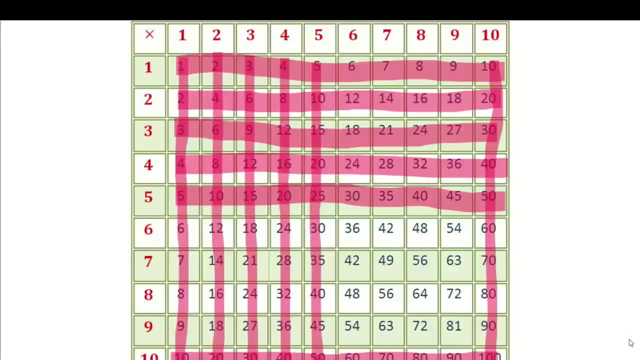 number to get the next number. And again, I'll always say what's five times five, Because it's the middle one, 25.. Once you've done that, You've really. The ones were easy, The twos were easy, The threes were easy, The fours were. 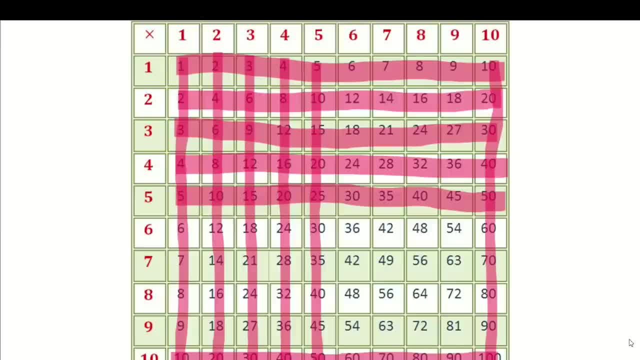 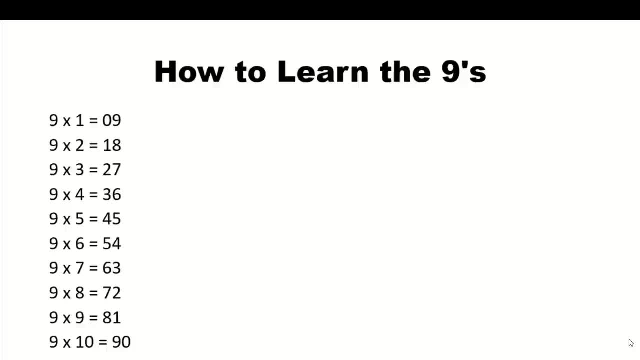 easy. The fives were easy. Now we are down to a four by four square here, And this is all we have to memorize. now How do you learn the nines? Nines are? There's a little bit of a trick to them. 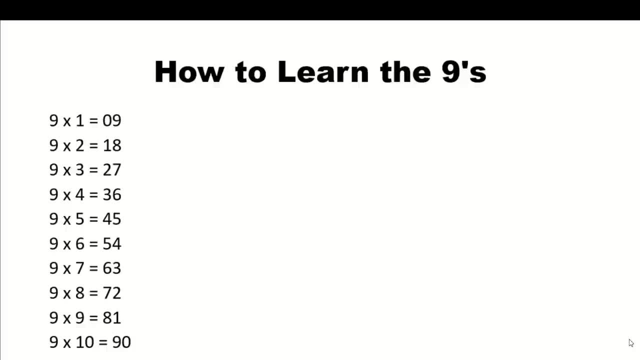 How do you learn the nines? Nines are? there's a little bit of a trick to them. that's kind of cool. If you do nine times one, you've got nine right, And I put zero nine there. But let's look at the next one. 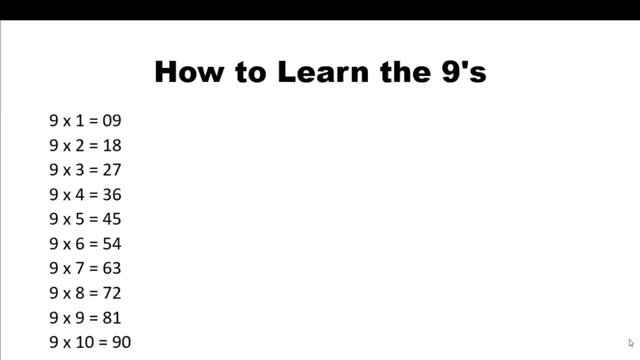 Nine times two is 18.. Well, what's one plus eight? It's nine. Nine times three is 27.. Well, what's two plus seven? It's nine. The answer in a multiplication problem: when you multiply a number by nine. 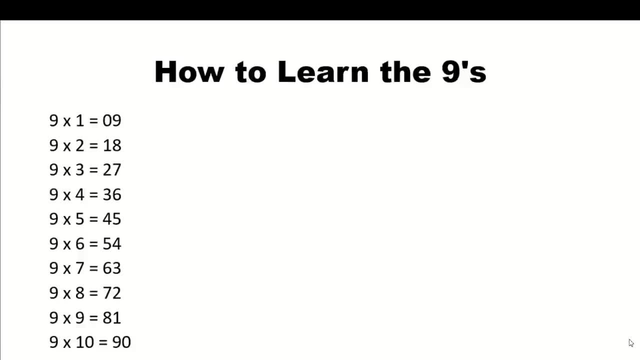 that's kind of cool. If you do nine times one, you've got nine right, And I put zero nine there. But let's look at the next one. Nine times two is 18.. Well, what's one plus eight? It's nine. 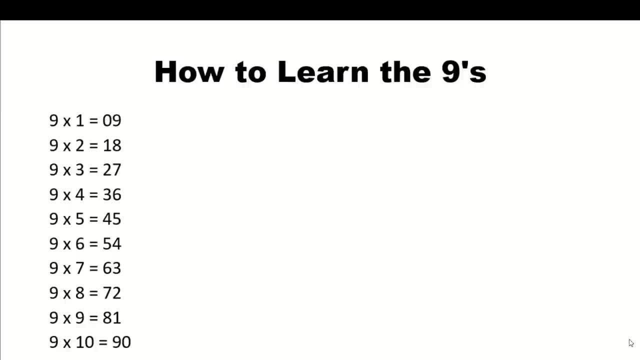 Nine times Three is 27.. Well, what's two plus seven? It's nine. The answer in a multiplication problem: when you multiply a number by nine, the digits add up to nine. Nine times four is 36.. What's? 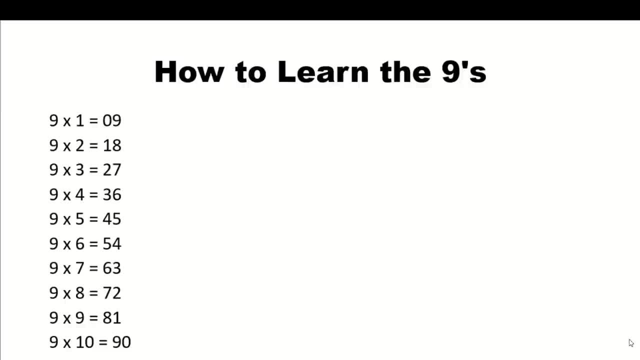 three plus six, It's nine. In other words, if your student is multiplying nine times four and they get an answer where the two digits don't add up to nine, they've done the math wrong. So tell them. this is a way to check their work. Nine times five is 44.. 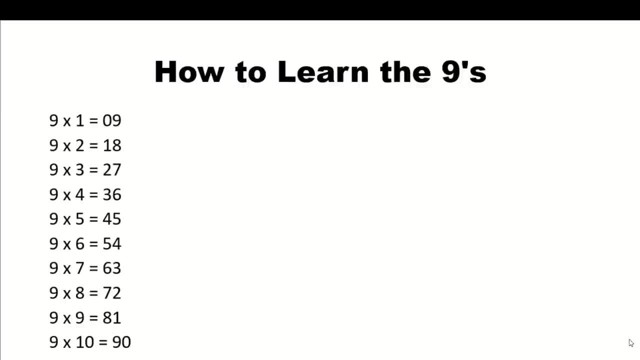 Four plus five is nine Nine times six is 54.. Five plus four is nine Nine times seven is 63.. Six plus three is nine Nine times eight is 72.. Seven plus two is nine Nine times nine is 81.. 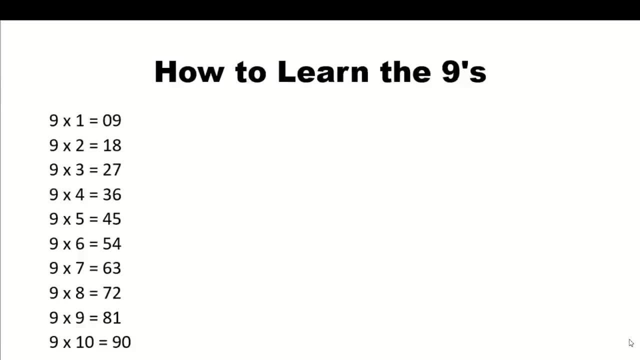 Eight plus one is nine, And nine times 10 is 90., And nine plus zero is nine. Now I'm going to show you another thing here on the nines. Look at this: Nine times two is 18.. The answer is always going to be one less than what you multiplied nine by. You multiplied nine. 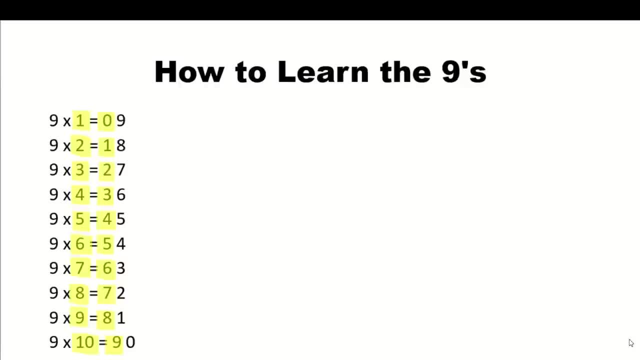 by two. What's going to be one less? It's going to start with a one. You multiplied nine times three. What's one less than three? It's two. Nine times four. What's one less than four? It's three. 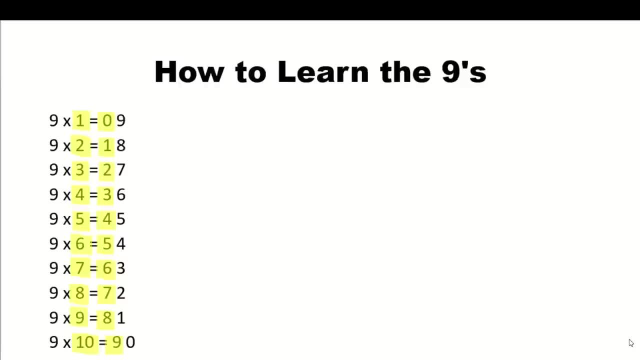 It's always. the answer is always going to start with one less than whatever. you multiplied by nine, Nine times seven, is 63.. What is one less than seven? It's six. So you know it's going to start with six. Now, what else do you know? 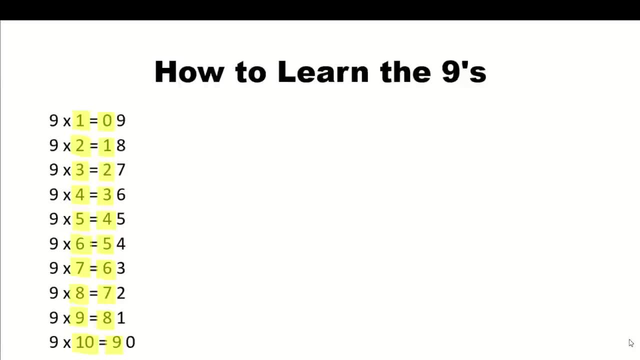 You know that it's always going to add up to be 9.. 6 plus 3 is 9.. 9 times 8 is 72.. 8, what's 1 less than 8?? It's 7.. What do you need to add to 7 to equal 9?? 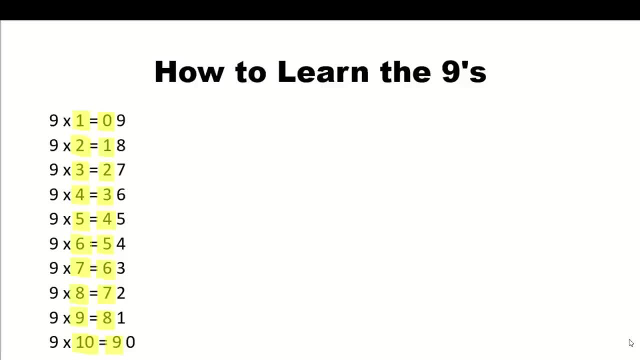 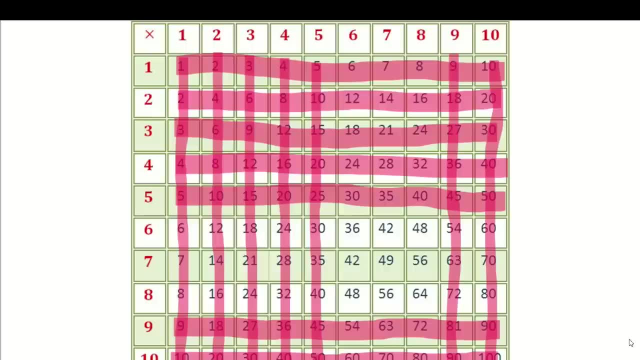 A 2. It's 72.. So 9s are real easy whenever you understand that the answer is always going to add up to 9.. So now you've crossed off the 9s and now you're down to a 3 by 3 square here. 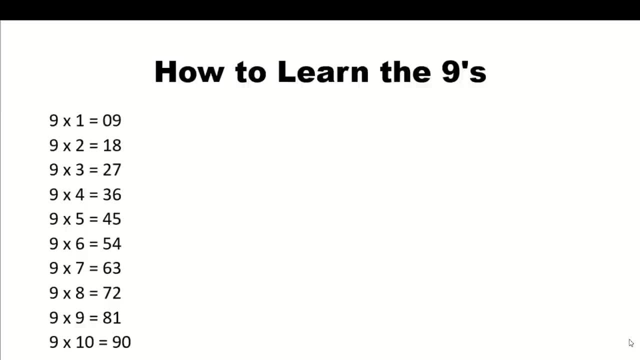 the digits add up to nine. Nine times four is 36.. What's three plus six? It's nine. In other words, if your student is multiplying nine times four and they get an answer where the two digits don't add up to nine, they've done the math wrong. 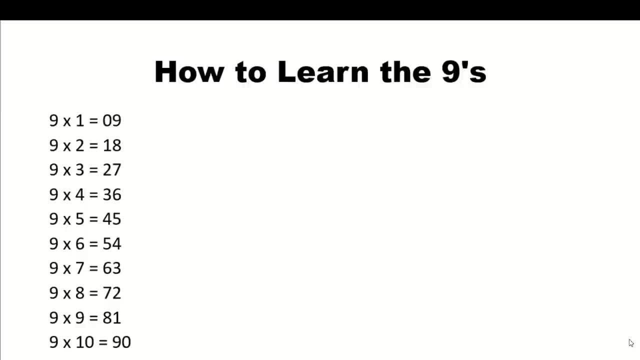 So tell them this is a way to check their work. Nine times five is 45.. Four plus five is nine. Nine times six is 54.. Five plus four is nine. Nine times seven is 63.. Six plus three is nine. 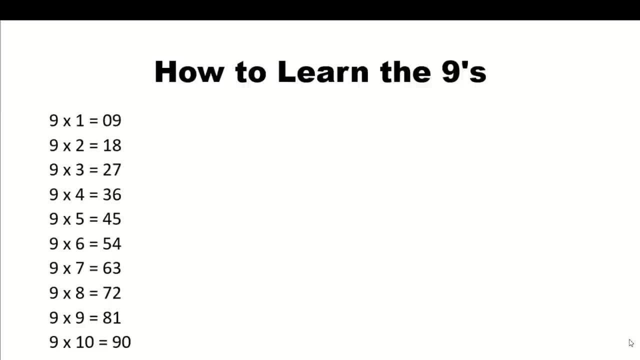 Nine times eight is 72.. Seven plus two is nine. Nine times nine is 81.. Eight plus one is nine, And nine times 10 is 90. And nine plus zero is nine. Now I'm going to show you another thing here on the nines. 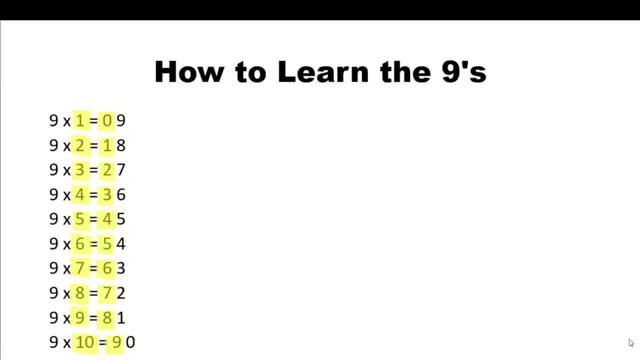 Look at this: Nine times two is 18.. The answer is always going to be one less than what you multiplied nine by. You multiply nine by two. it's going to be one less. It's going to start with the one You multiply nine times three. 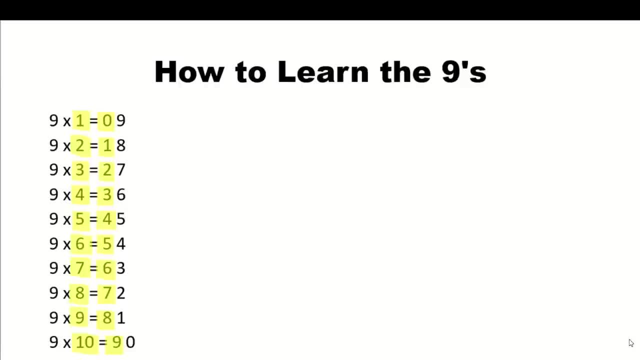 What's one less than three? It's two. Nine times four. What's one less than four? It's three. The answer is always going to start with one less than whatever. you multiplied by nine Nine times seven is 63.. What is one less than seven? 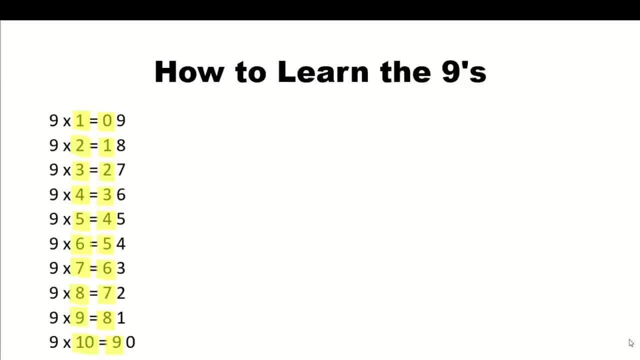 It's six. So you know it's going to start with six. Now, what else do you know? You know that it's always going to add up to be 9.. 6 plus 3 is 9.. 9 times 8 is 72.. 8, what's 1 less than 8?? It's 7.. What do you need to add to? 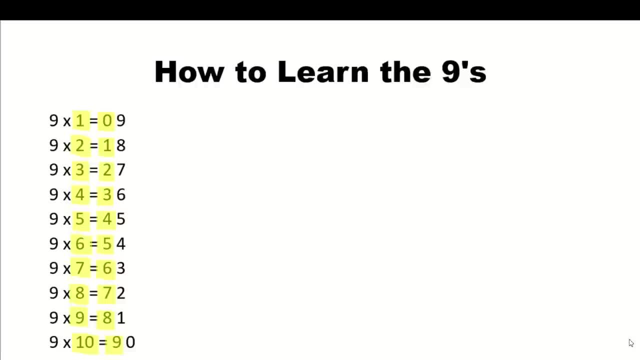 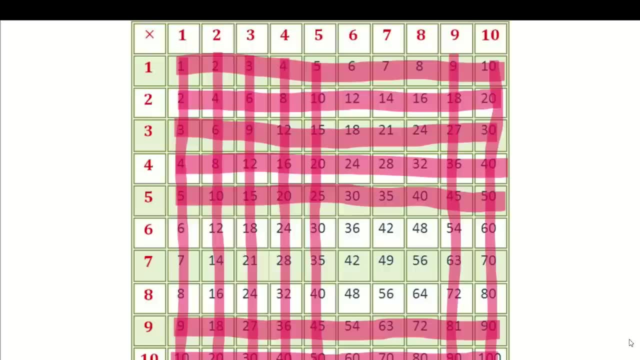 7 to equal 9? A 2. It's 72. So 9s are real, real easy. whenever you understand that, the answer is always going to add up to 9.. So now you've crossed off the 9s, and now you're down to a 3 by 3. 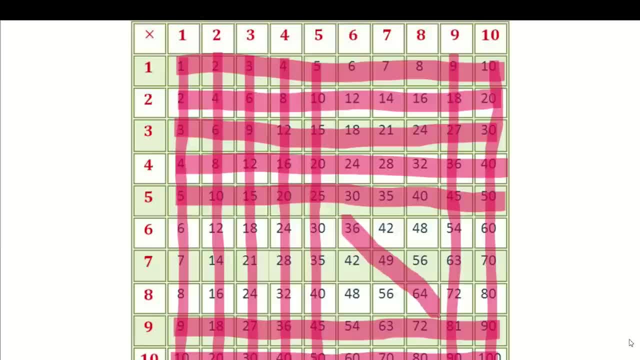 square here. This is really all you got to memorize. Now, people find the squares of numbers sometimes easy: 6 times 6 is 36.. 7 times 7 is 49.. 8 times 8 is 64.. For whatever reason, people just. 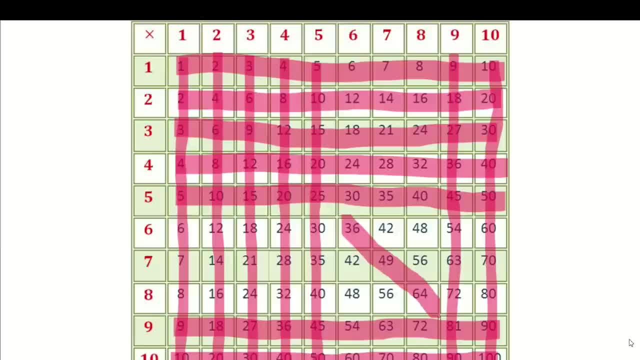 This is really all you've got to memorize. Now, people find the squares of numbers sometimes easy: 6 times 6 is 36.. 7 times 7 is 49.. 8 times 8 is 64.. For whatever reason, people just tend to kids, tend to get those and understand those quicker. 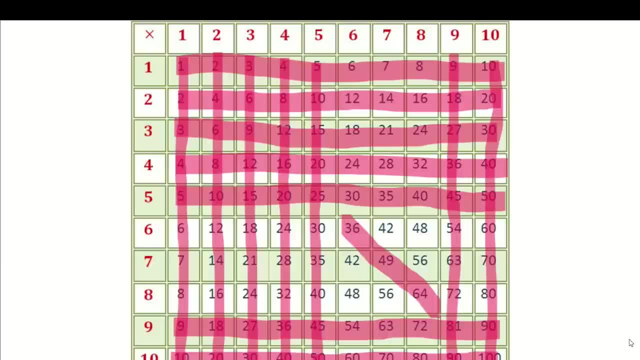 So now we're left with 6 answers here, or 6 different squares, but that's just 3 different multiplication problems. You have 7 times 6, you've got to learn it's 42.. You've got to learn that 6 times 8 is 48.. 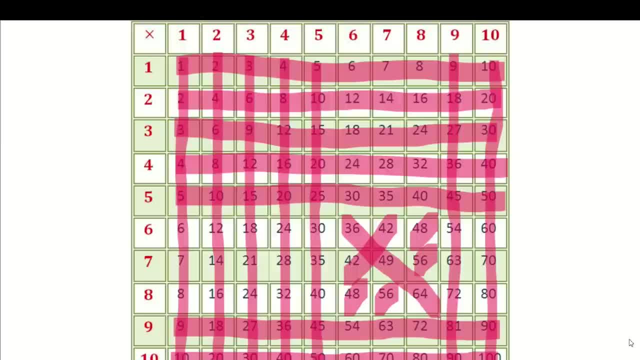 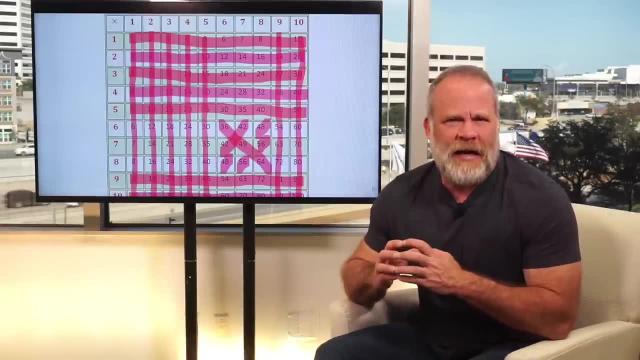 And you have to learn that 7 times 8 is 56. So really those last 3 are really the only 3 challenging ones. But here's the deal If you're trying to teach a student how to memorize the multiplication tables, 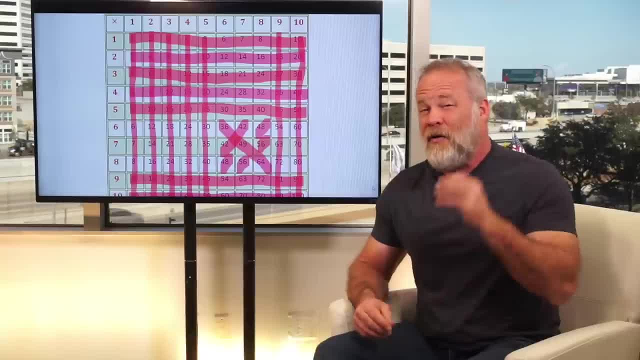 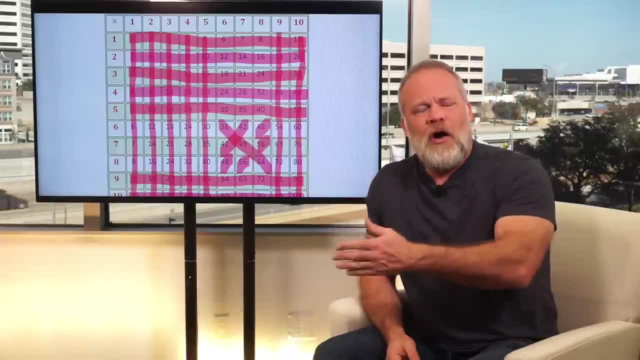 break it down like this and go through each one. And when you go through each one, you're going to end up realizing: hey, this wasn't that difficult at all. But you know what? Learning isn't difficult at all when you approach it in the right direction. 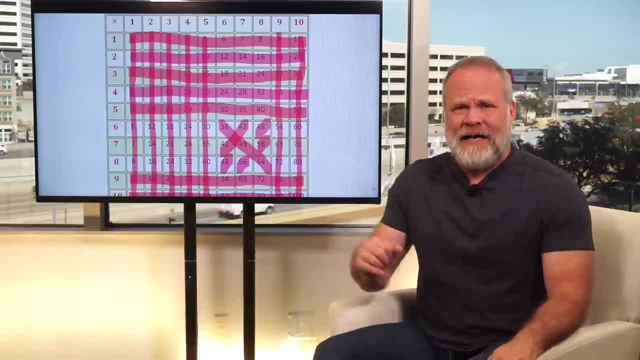 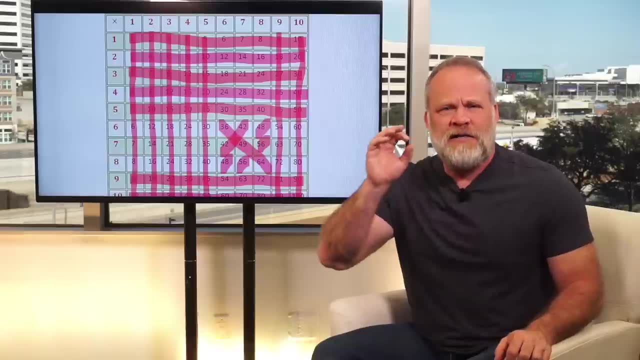 That's why I created my Black Belt Memory course. If you click the link down below, you're going to see I'm going to show you how to dismantle anything you're trying to learn in the same systematic way: What you read, studying for a test, languages, whatever you want to learn. 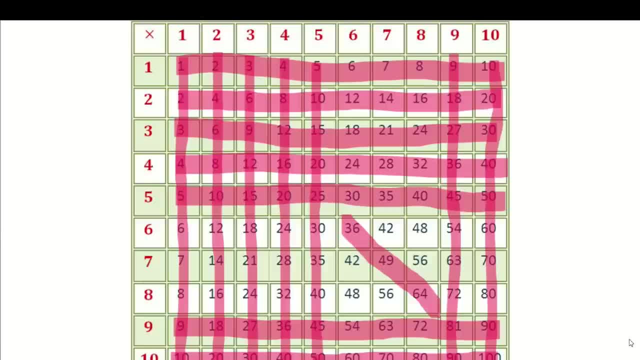 tend to. kids tend to get those and understand those quicker. So now we're left with 6 answers here, but 3 or 6 different squares, but that's just 3 different multiplication problems. You have 7 times 6, you got to learn it's 42.. You've got to learn that 6 times 8 is. 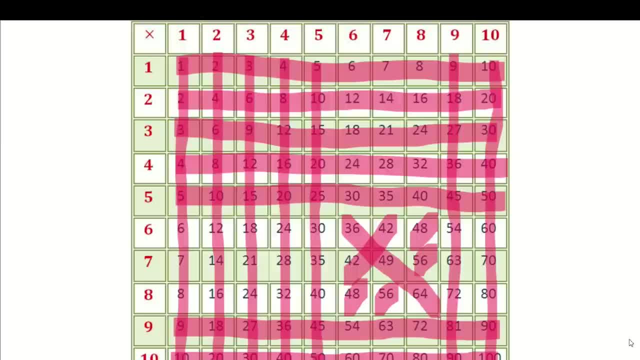 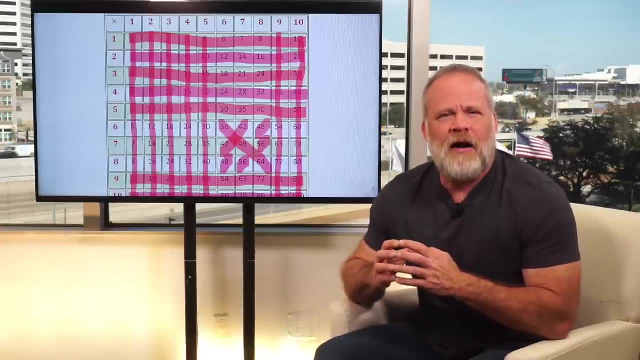 48, and you have to learn that 7 times 8 is 56. So really, those last three are really the only three challenging ones. But here's the deal: If you're trying to teach a student how to memorize the multiplication tables, break it down by like this and go through each one, And when you go, 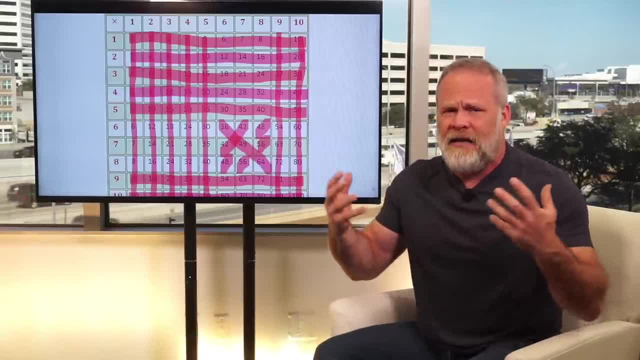 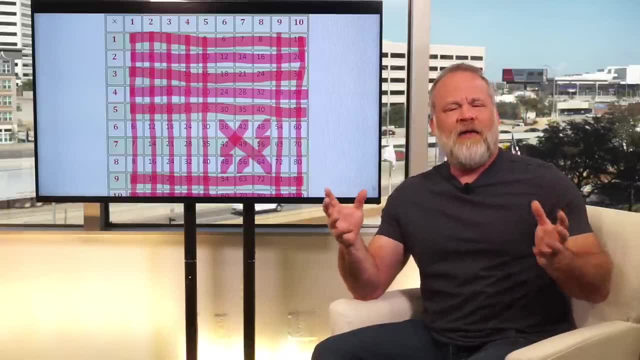 through each one, you're going to end up realizing: hey, this wasn't that difficult at all. But you know what? Learning isn't difficult at all when you approach it in the right direction. That's why I created my Black Belt Memory course. If you click the link down below, you're going to 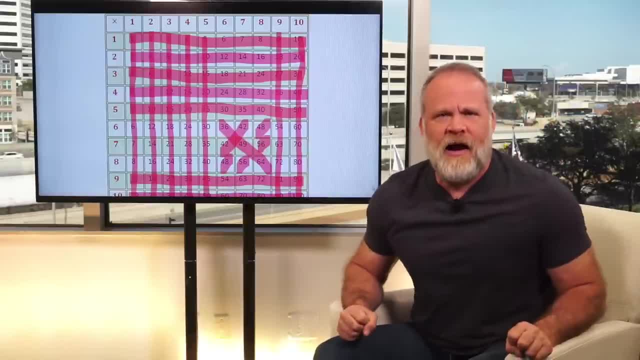 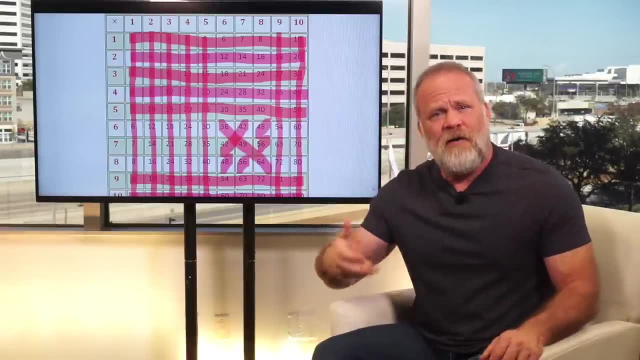 see, I'm going to show you how to dismantle anything you're trying to learn in the same systematic way: What you read, studying for tests, languages- whatever you want to learn, you can learn it faster with my course. Click the link down below If this multiplication video helped. 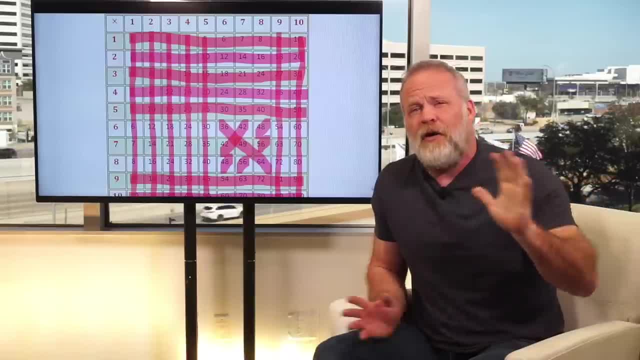 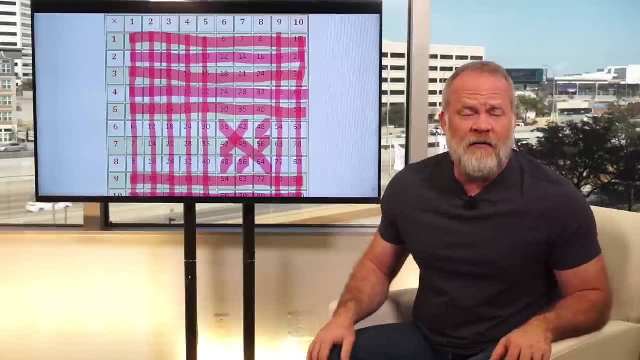 you and helped your kids. I would love the thumbs up. I would really appreciate that, But also comment down below and tell me what you or your kids are working on and studying, and maybe I can help create a video for that. Do not forget to subscribe and I'll see you on the next one.